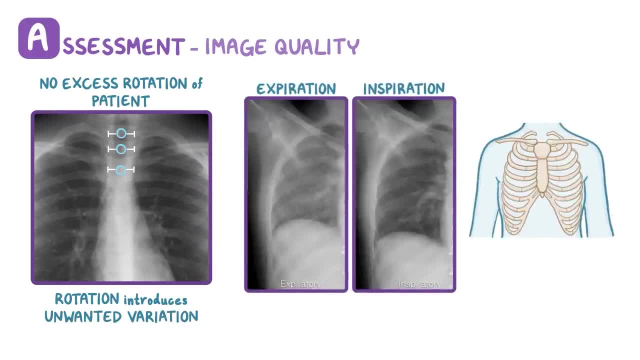 Next, a good inspiration film should show at least the 10th or 11th posterior ribs. If the lungs are not fully expanded, we might miss important diseases. Finally, we need to make sure that the exposure isn't too bright or too dark To check for. 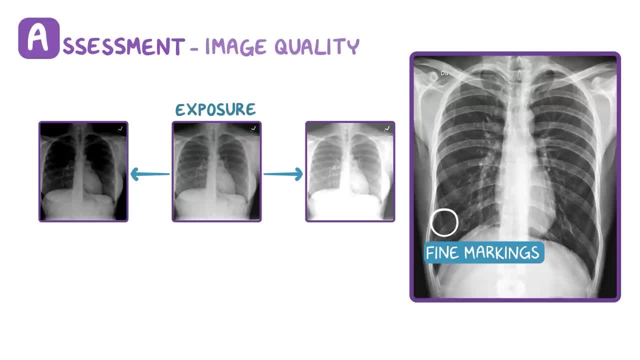 this. you can look for fine markings in the lung fields to make sure they're visible. If the fine lung markings aren't visible, then the X-ray may fail to detect some diseases. A also reminds us to make sure there isn't air where it shouldn't be, Finding air where. 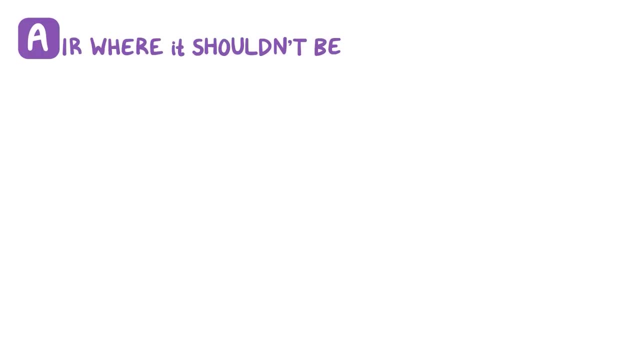 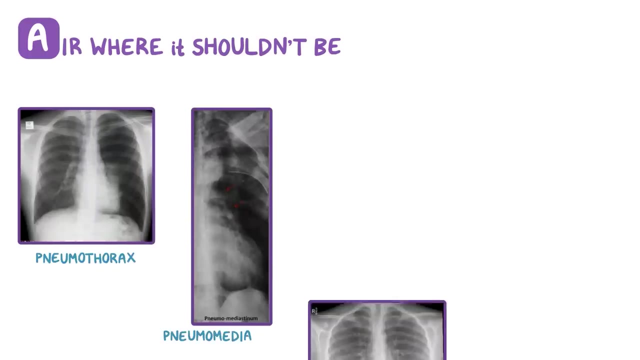 it should not be, or, more commonly, ruling it out, remains one of the most important uses of medical X-rays Diagnoses like pneumothorax, pneumomediastinum, pneumoperitoneum and subcutaneous. 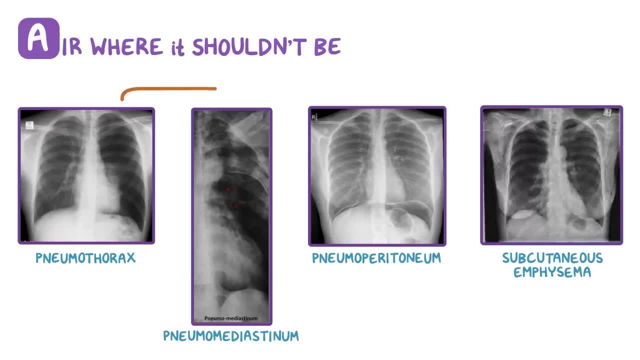 emphysema are all examples of air where it shouldn't be. Thanks for watching. All of these are surgical emergencies and can be diagnosed by a simple chest X-ray. Finally, if the major airways, like the trachea, are bent or deviated- another example of air. 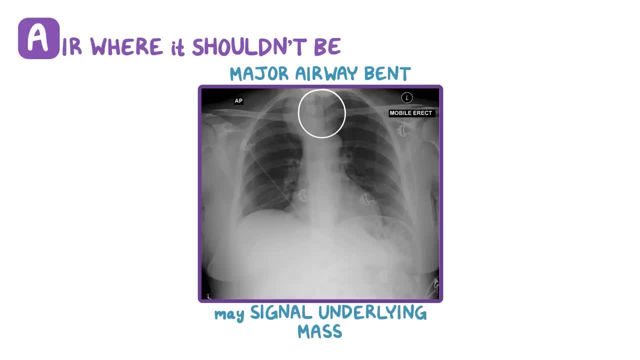 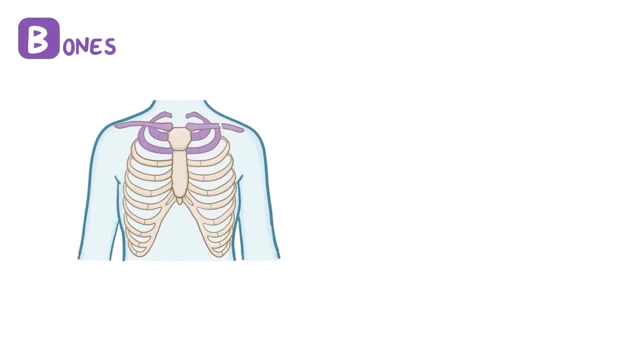 where it shouldn't be. it may signal an underlying mass. B is for bones. Start by looking at both clavicles and all 12 pairs of ribs, one at a time, to make sure that there are no fractures, deformities or missing bones. B is also for the lungs. If the lungs are not fully expanded we might miss important diseases. H is for the reflex leaving the body and L is for improper organWhich is the exc resting fought area, especially in post-express tonics. 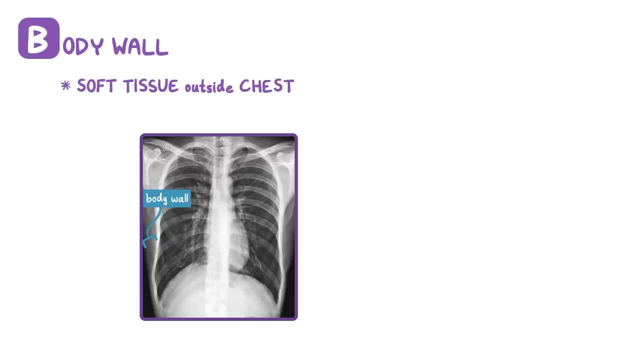 C is for the around the abdomen. B, if the particularly large strabismus muscle up by weight. Jaumer is the ideal base for spleen breaks or the rough dry Emerald. H is for constituents like growthân Cyst as another example. 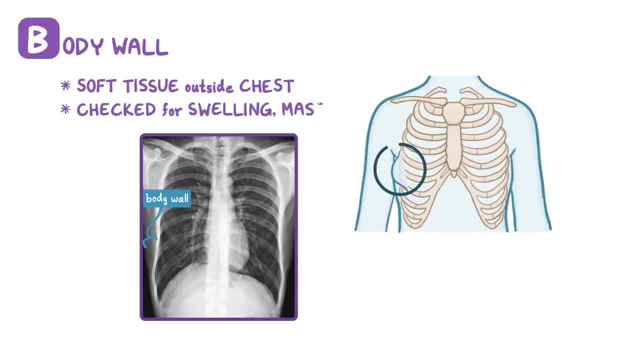 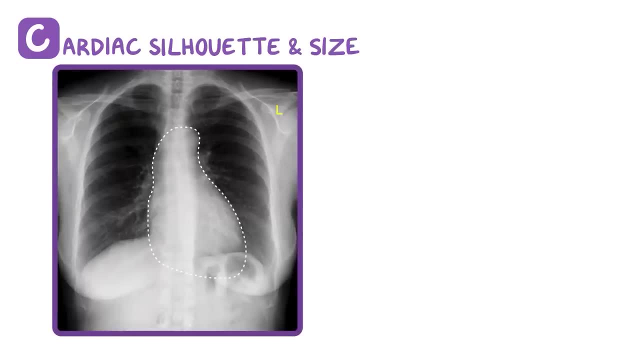 B is also for the body wall And soft tissues outside of the chest. C is for cardiac silhouette and size. This is the familiar cardiac silhouette: atder space, atada space, And there is an atrial appendage, the right atrium. 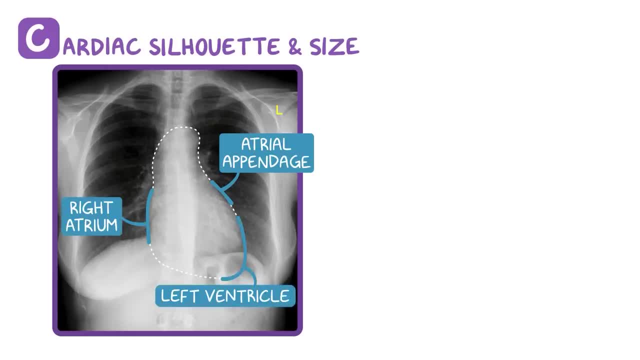 and the left ventricle. Remember, in chest X-rays we define features relative to the patient. so the right atrium is on the left side of this X-ray and the left is the tearing. we define the opponent's top facing augment tatum and the lowerrium. 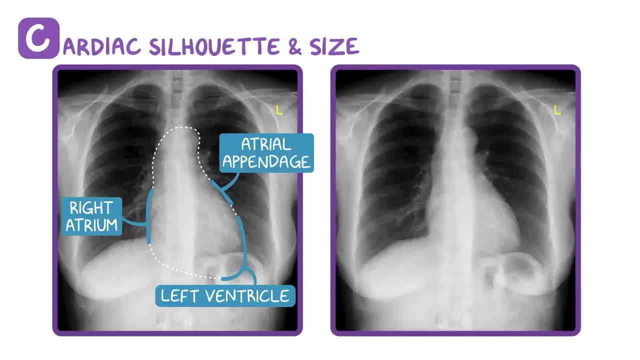 this x-ray and the left ventricle is on the right side. Measuring across a normal heart is less than 50% of the greatest diameter of the rib cage measured from the inner portion of each rib. Any larger and there may be cardiac pathology. 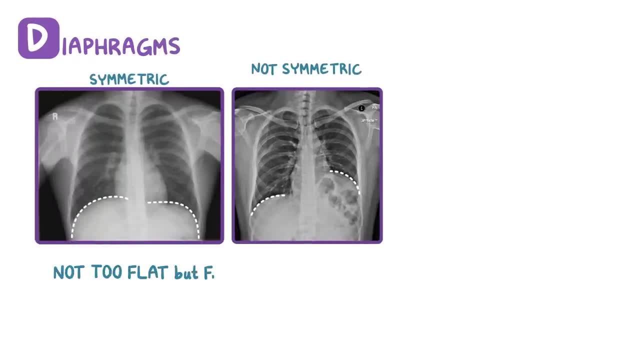 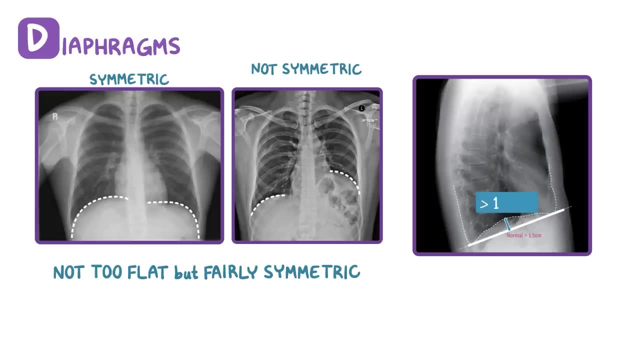 D is for the diaphragms, which shouldn't be too flat but appear fairly symmetric. You can assess flatness on the lateral view by estimating that the hemidiaphragm is 1.5 cm above the line connecting the costophrenic angle posteriorly and sternophrenic angle. 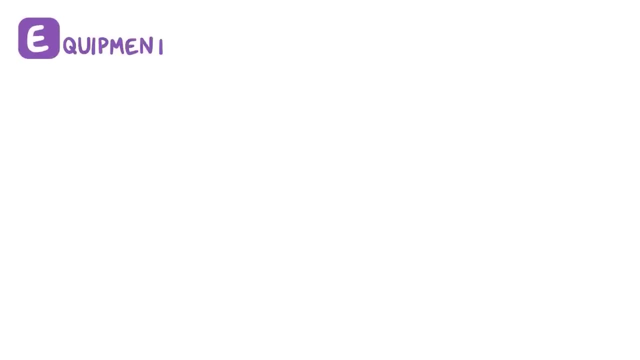 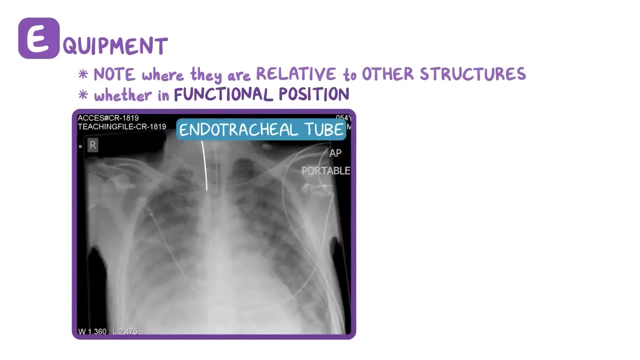 anteriorly. E is for equipment such as lines, tubes and wires involved in life support. It's important to note exactly where they're located relative to other structures and whether they're in functional position. For example, an endotracheal tube should be in the middle of the trachea and its tip. 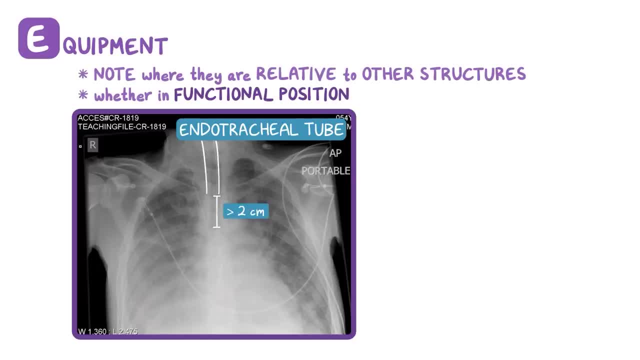 should be more than 2 cm from the tracheal bifurcation Or if the endotracheal tube is in the middle of the trachea. the endotracheal tube should be more than 2 cm from the trachea and its tip should be more than 2 cm from the trachea. 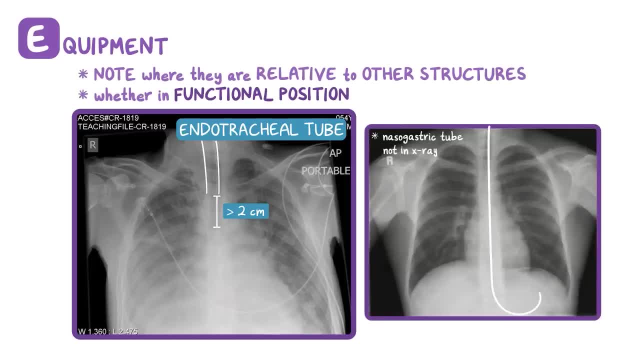 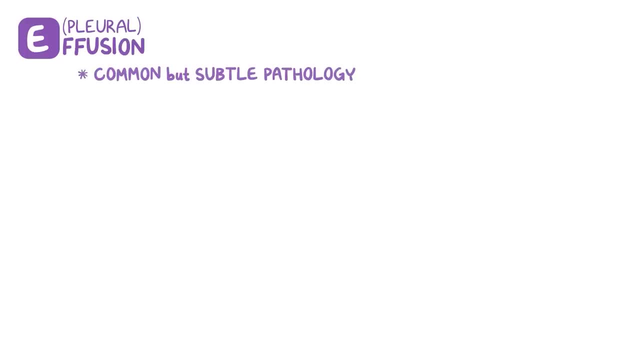 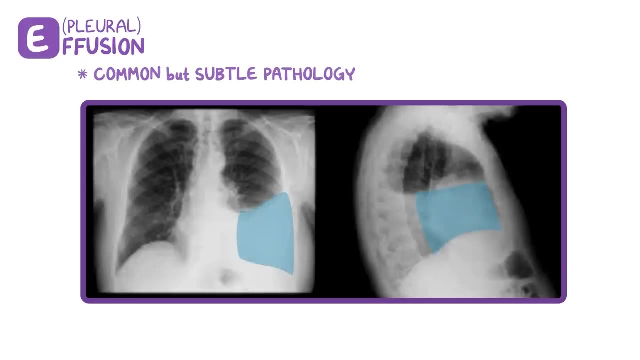 Or that a nasogastric tube should have its tip well within the stomach. E is also a reminder to check for a pleural effusion, which is a common but subtle form of pathology that you can see on an x-ray. Pleural effusions are fluid that collects at the costophrenic angle and causes blunting. 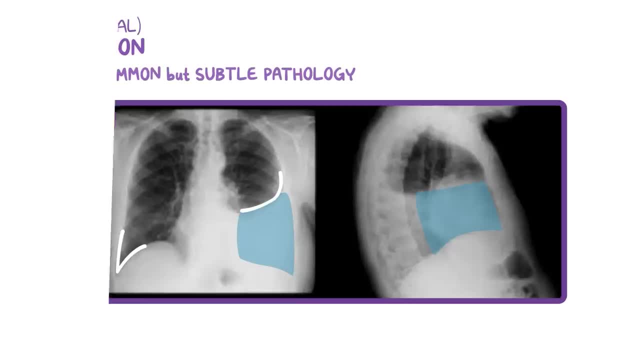 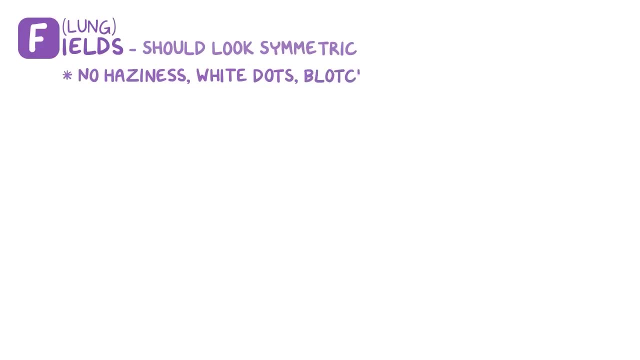 of the normally sharp costophrenic angle F is for lung fields, which should look symmetric. There shouldn't be any haziness, white dots or blotches. While looking at lung fields, having a frontal and a lateral x-ray allows us to determine. 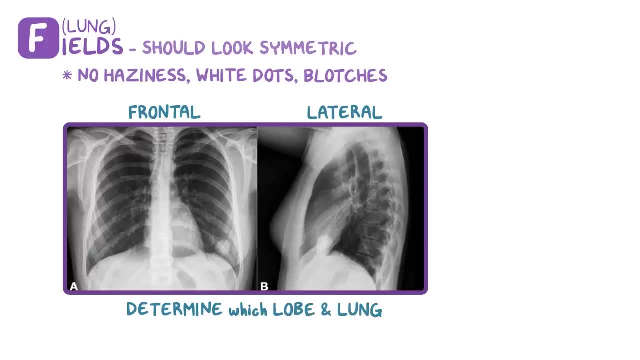 in which lobe of which lung an abnormality is located. In this case, a nodular mass is visible in the inferior, lateral and anterior left lung, meaning it's most likely within the anteromedial basal subsegment of the lower left lobe. 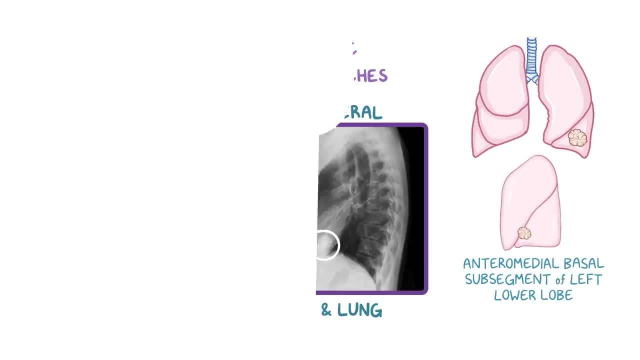 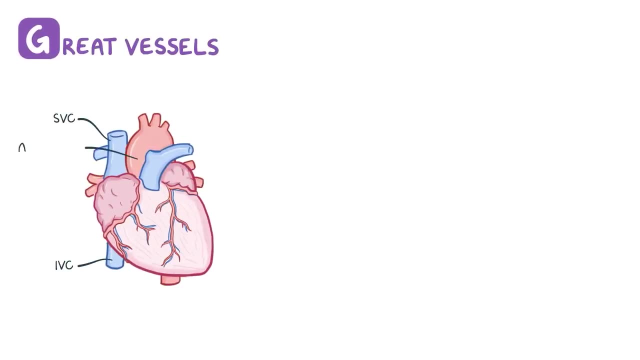 This can be confirmed with a chest CT. Lastly, G is for great vessels. This includes the superior vena cava, inferior vena cava, ascending aorta, aortic arch, pulmonary artery and descending aorta. You want to make sure that all of these structures are in the right location and is the right.